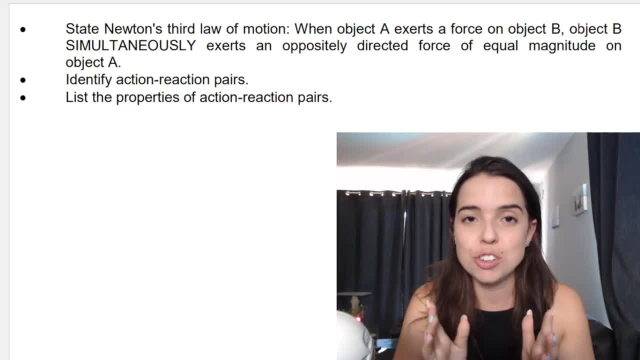 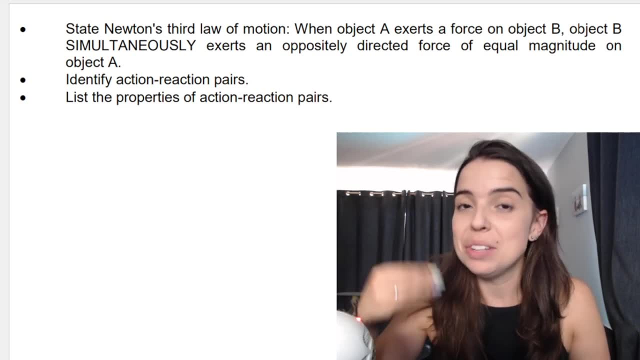 all that the exam guideline states on Newton's third law of motion. So there's a definition. They say that you must be able to identify action reaction pairs and list properties of these pairs. So first things first. what is Newton's third law of motion? Well, the definition of Newton's third law. 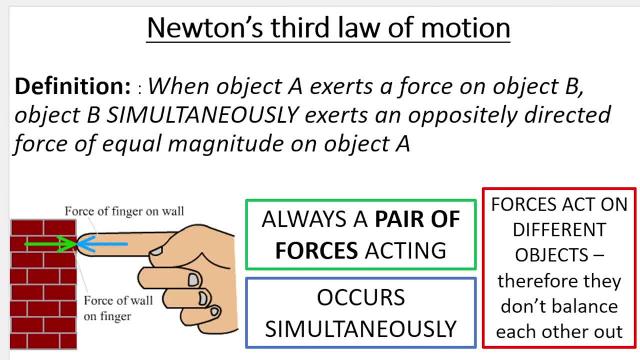 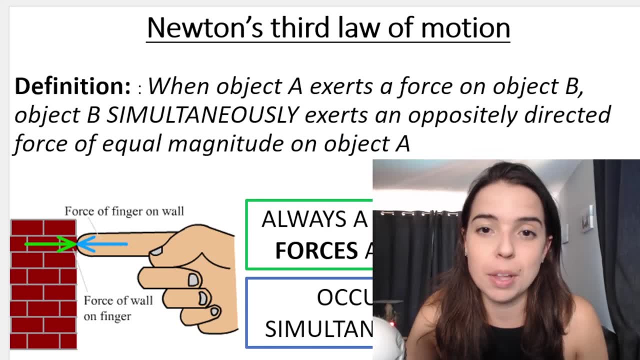 of motion says: when object A exerts a force on object B, object B simultaneously exerts an oppositely directed force of equal magnitude on object A. Now that's a mouthful, but if we break it down it's as simple as this. So let's take a look at the diagram over there. So finger on. 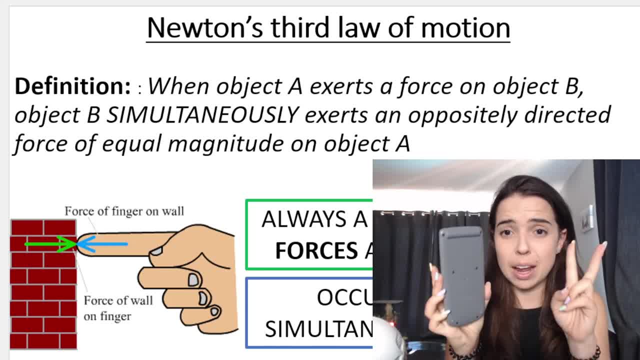 what is the force on object B? So if we break it down, it's as simple as this. So let's take a look at the wall diagram. I will use my calculator is my wall and here's my finger. So when object A 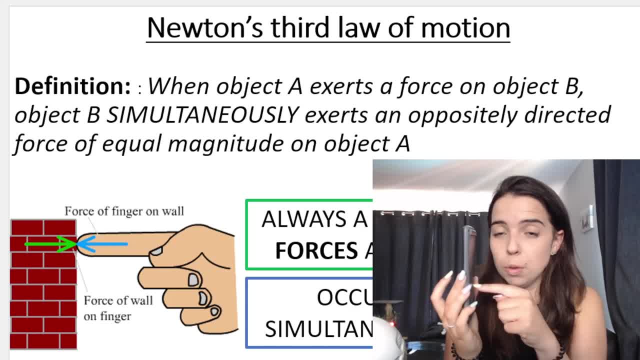 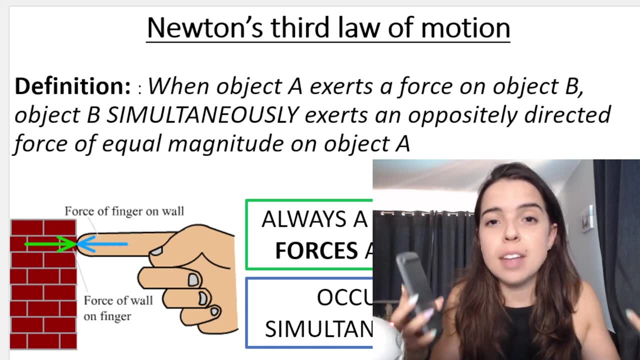 my finger exerts a force on object B, my wall, Object B simultaneously, which means at the same time, at the exact same time, exerts an oppositely directed force. So force going in the opposite direction, of equal magnitude, which means the same size, on object A. So if my finger exerts a force, 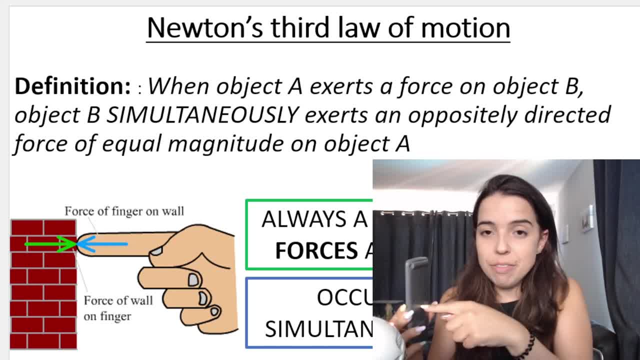 of 20 newton per second, I will exert a force of 20 newton per second. So if my finger exerts a force to the left on the wall 20 newton left is finger on wall. my wall exerts 20 newton to the right on. 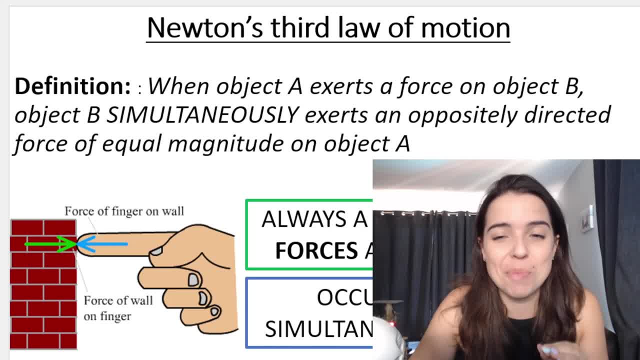 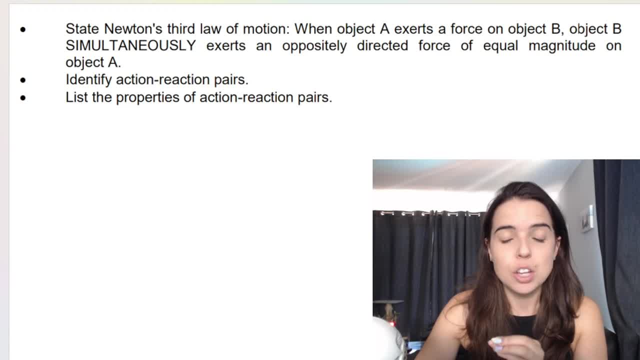 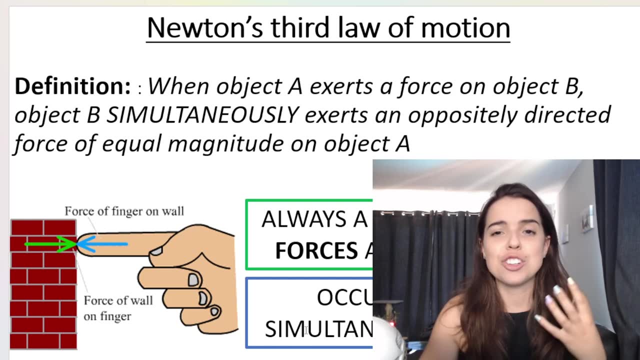 my finger. Okay, so that is basically all that Newton's third law of motion is saying. What's important to note? remember we discussed the properties of action-reaction pairs. So finger and wall, that is my action-reaction pair. or it can be book and desk, that is my action-reaction. 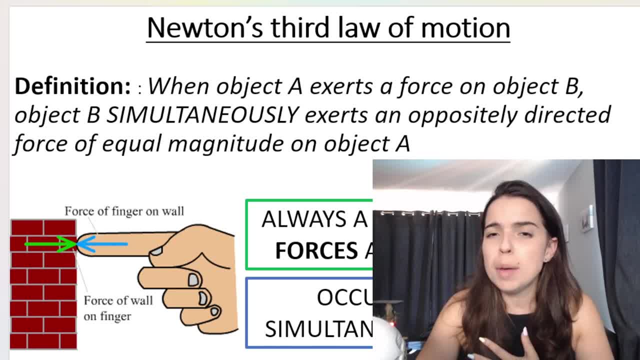 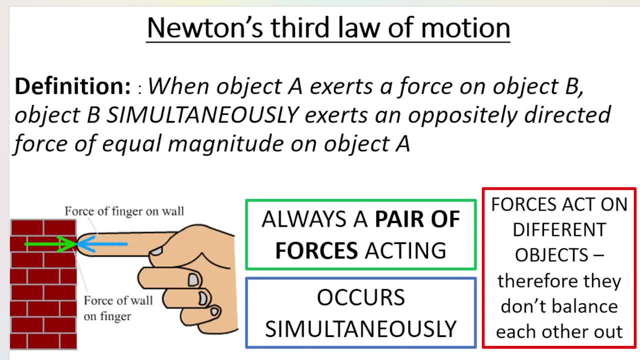 pair. There's always two things in a pair, So the properties of action-reaction pairs are the properties. what do I mean by properties? Well, first of all, the forces are always acting in pairs, So that's why it says you're always a pair of forces acting. It occurs simultaneously, which 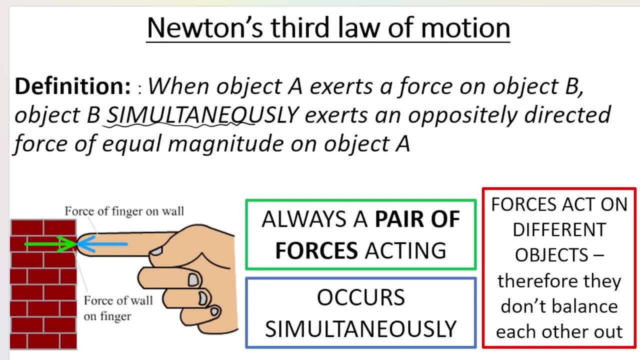 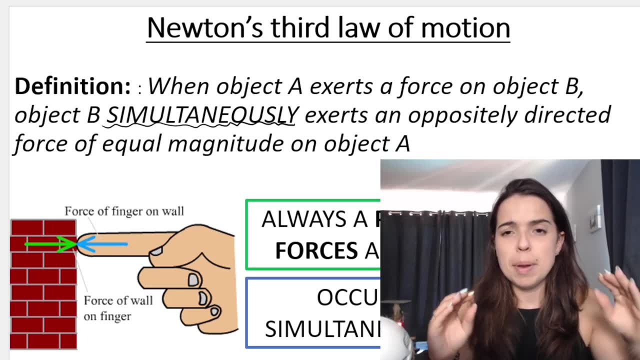 means at the exact same time as the definition states. it even states it in capital letters. And the forces act on different objects. therefore they don't balance each other out. Now, this is what is so important to understand. A lot of people don't understand this concept. They're saying: but 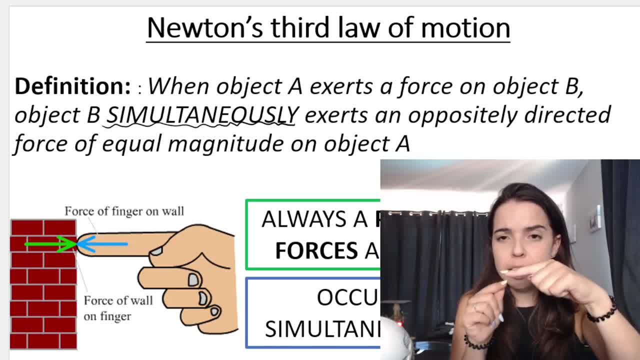 let's imagine: if you've got your finger on the wall and your wall on your finger, How can you push something over? Don't the forces cancel each other out? The forces will only cancel each other out if they're acting on the same object, But for Newton's third law of motion, the forces will. 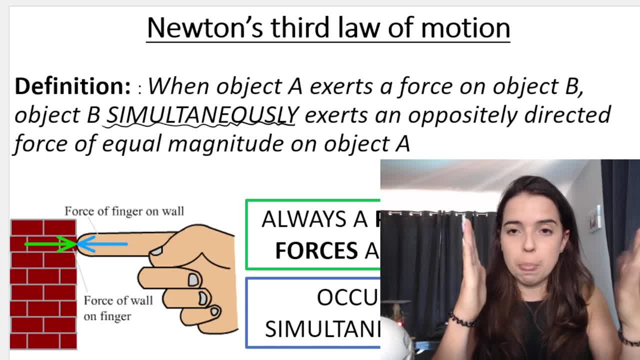 act on different objects. So if we have, like, let's say, a pen on hand, The one force is acting on the pen, The other force is acting on the hand. So because the two forces worked on one hand, the pen becomes another strength of action, Isn't it? The few other forces are acting on the other team. soda or aguru? Does candy still remain the same? If you make use of the two forces, what is your diamond? And then from there, if you take the chi, I'll call it corner. so there'sουμεin so many. 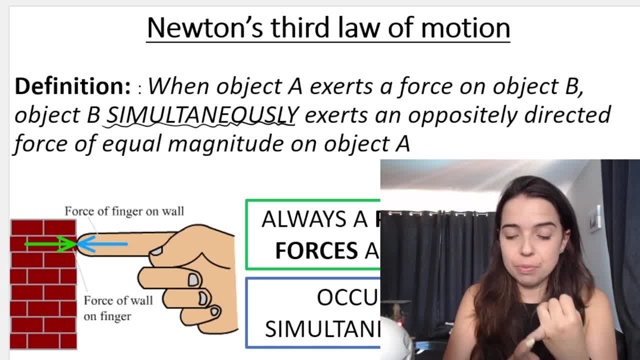 Because the two forces play different implications. The superann Na giShow is much complete, whereas the three, the two forces. i know they're equal in magnitude, that means that they're the same size. i know they're opposite in direction, but because they're on different objects they don't balance or cancel. 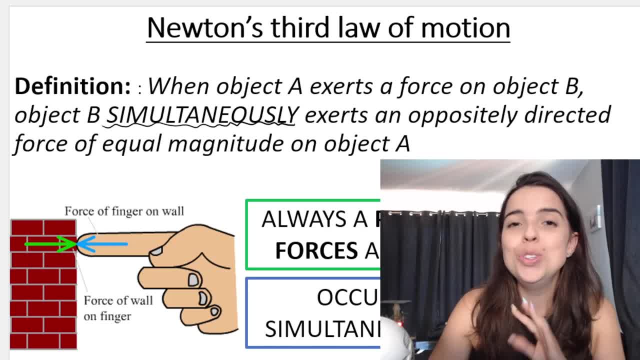 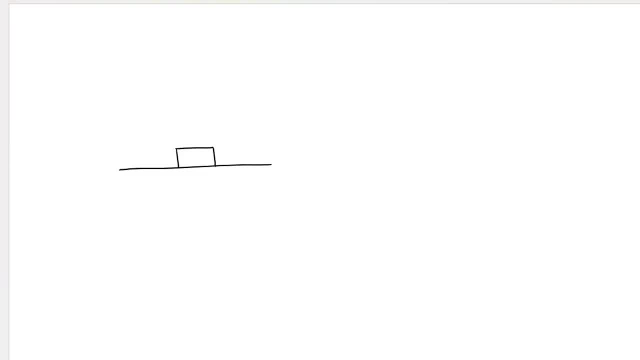 each other out. okay, it's super important to understand, super, super, super important. so if we take a look at some examples where some people often go wrong- now this is very important- is say, i have a box lying on a table. some people want to tell me that the weight of that book, let's call. 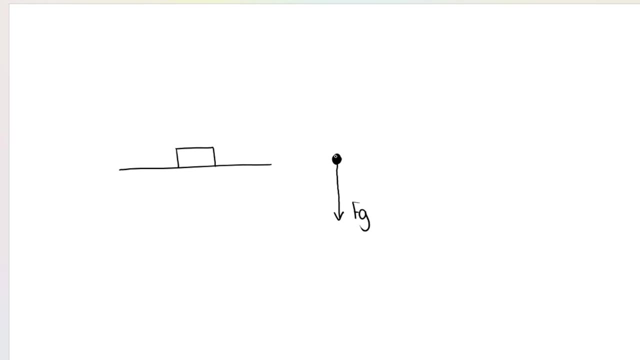 it a book. let's call it fg, which is the weight of the book. they want to tell me that the newton's third law, the action reaction pairs, is the normal force. that is not true. that is not true, remember, if you consider the weight of an object and the normal force of an object, the weight of the object. 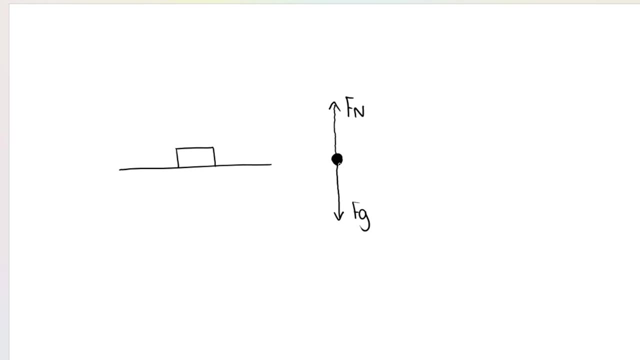 acts on the object to the weight of the book. this fg. it acts on the book. the normal force is the force that the table exerts on the book. so normal force and fg are on the same object. that's why we draw them on the same free body diagram. yeah, they're both acting on the dot and remember, the dot is now my. 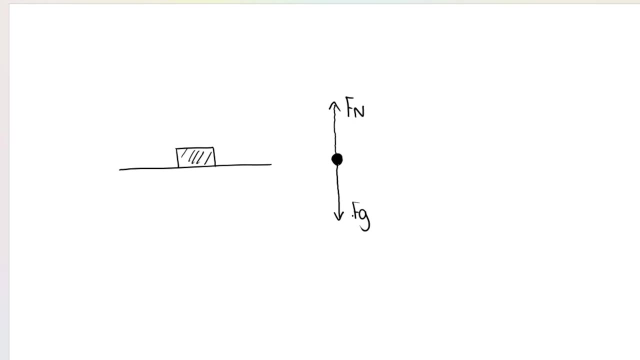 book or my object. this is not an example of newton's third law of motion. if i had to ask you, what is the newton's third law of motion? action, reaction pairs that correspond to the normal force. think about the normal force. the normal force is the, the force of the table. 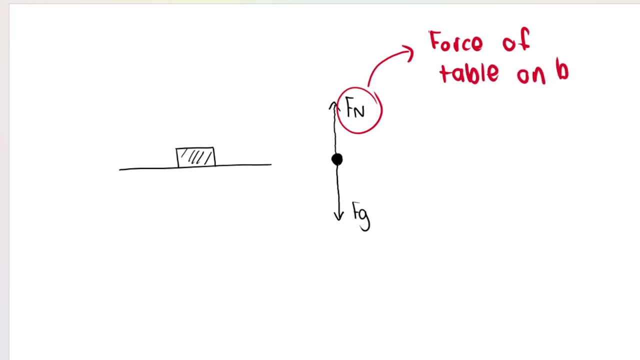 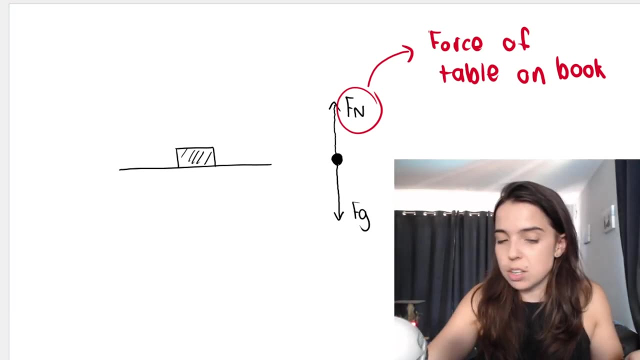 on the book, right, the force that the table exerts on the book. that is what the normal force is. remember, here's my table, here's my book. the normal force is the force exerted by, the force exerted on the book, by the surface on with which the object is in contact with. so the normal force would be: 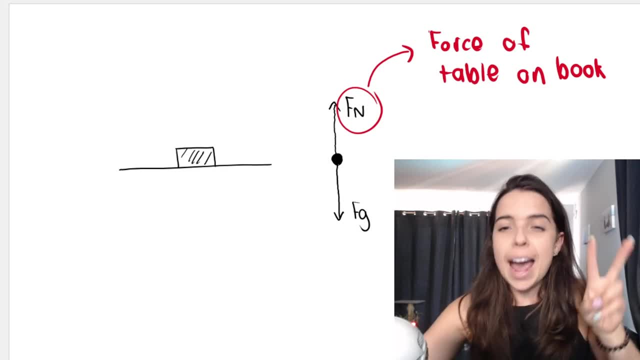 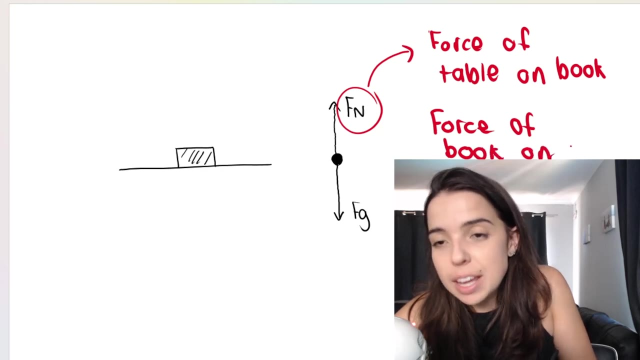 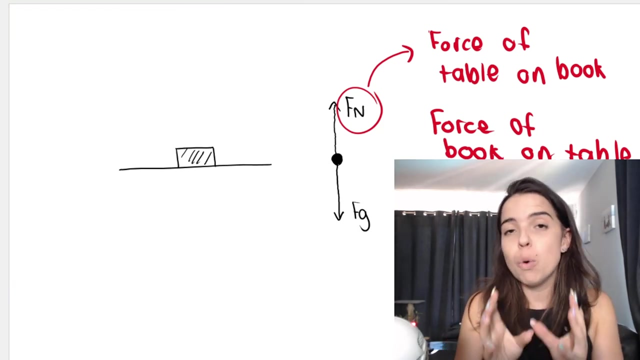 my force of my table on my book, the action reaction pair. so the pair of that force would be the force of the book on the table, the force of the book on the table, and that's not the same thing as the weight, the weight, the force of the weights. 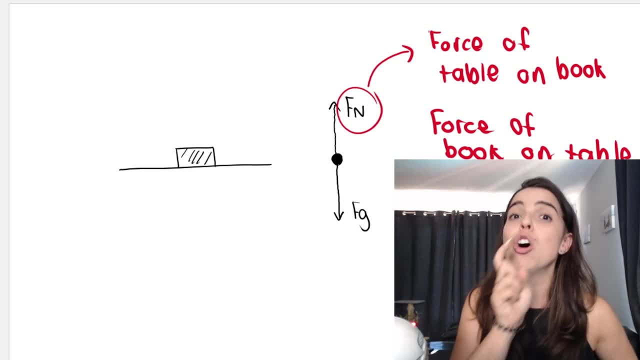 fg. what fg is? that's the force of the earth on the book. so do you see how i'm mentioning completely separate objects? so the normal force is the force of the table on the book. its action reaction pair would be the force of the book on the table. so i just reversed the words. 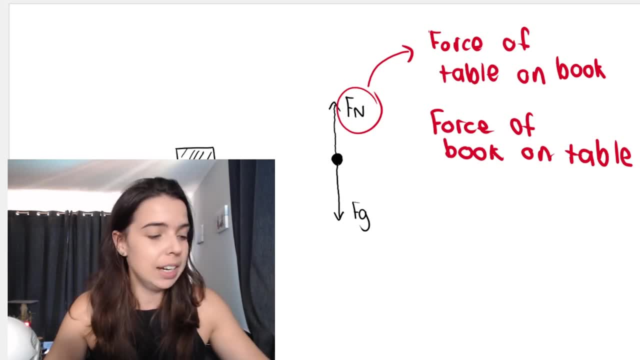 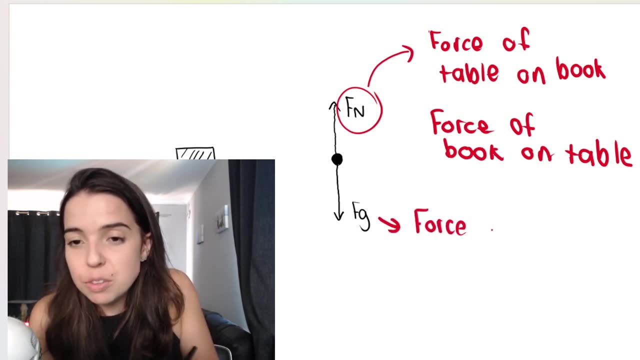 if i look at the weight. however, let's take a look at weight. what is weight? you guys should know what weight is. weight is the force- we just said it. it's the fourth force that the book is- the earth exerts on the book. so the weight of a book, that's the force that the earth exerts on. 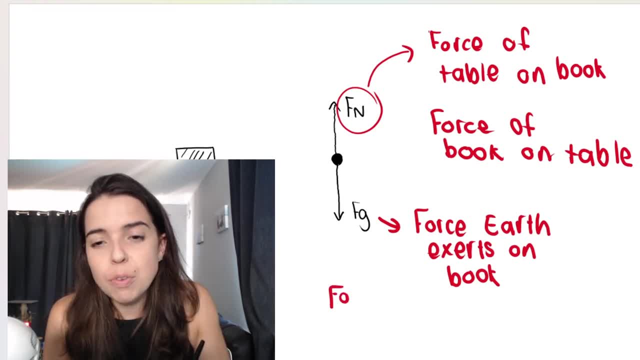 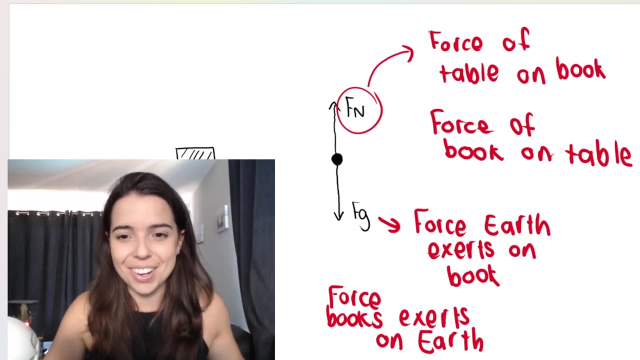 the book, what is its action reaction pair? it'll be the force that the book exerts on the earth. okay, and that's weird, you're probably like huh, the book is exerting a force on the earth, so the book is pulling the earth up? yeah, it is. those are actions that the book is pulling. 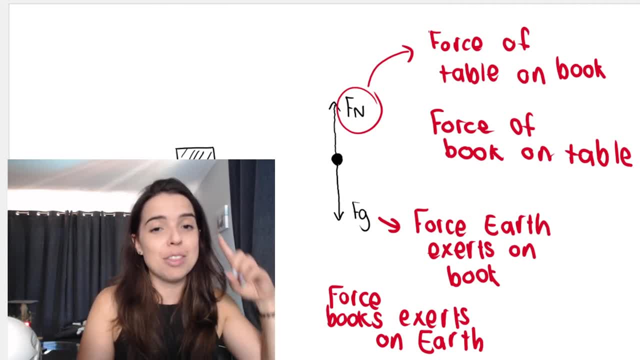 action reaction pairs. so please don't make the mistake of telling me that the normal force and fg are an example of newton's third law of motion. they're not. they're acting on the same object and, as we just said in the previous little picture over here, that the forces act on, 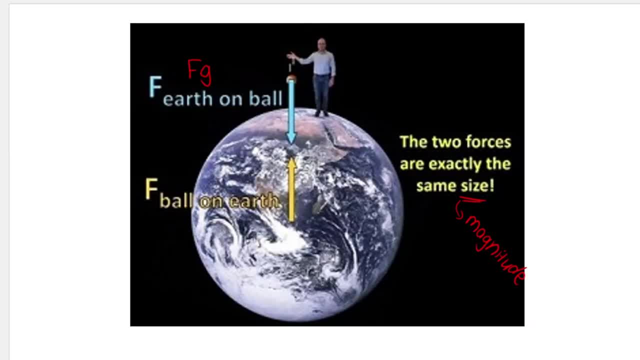 different objects. okay, so here's another example of newton's third law of motion. so the force of the earth on the ball, that is called the weight, that is called the weight of the ball, or Fg, the force of earth on the ball. And the force of the ball on the earth would be its action. 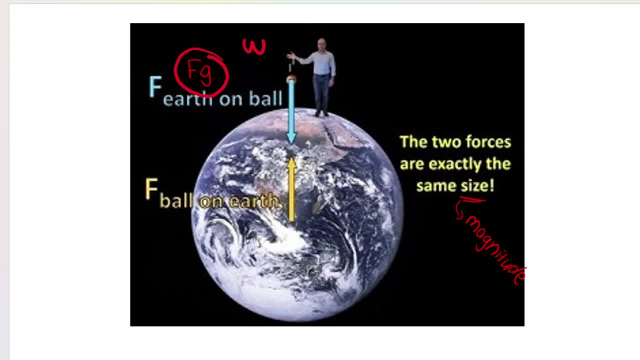 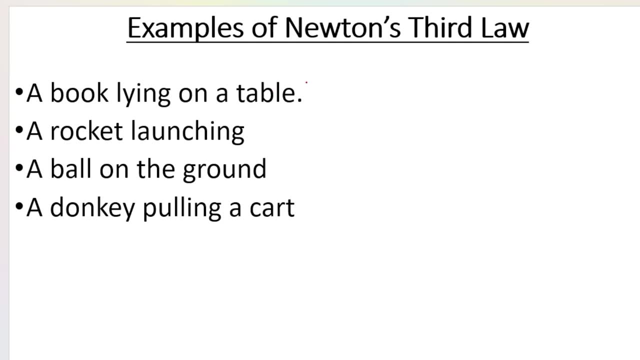 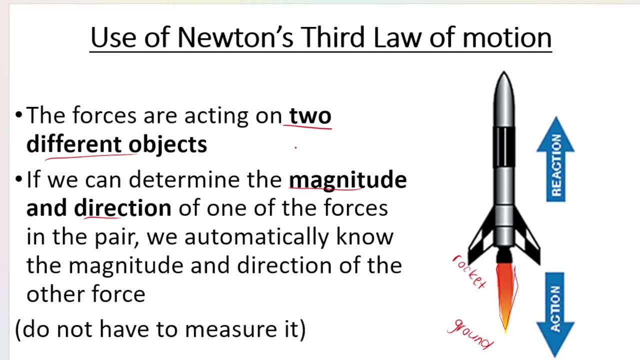 reaction pair. They have the same size, same magnitude. So if you had to do this one- the force of the book, the force of the table on the book and the force of the book on the table- that would be an action reaction pair. They act on different objects. So what this means is, if we know the 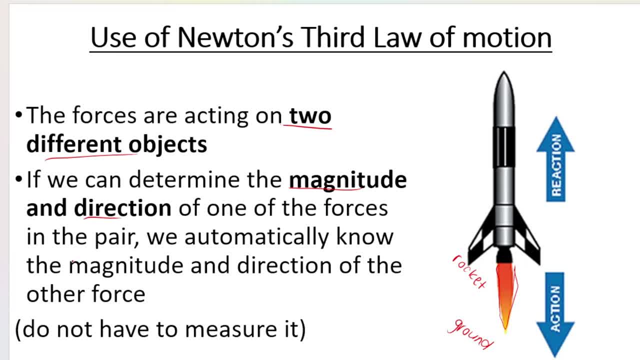 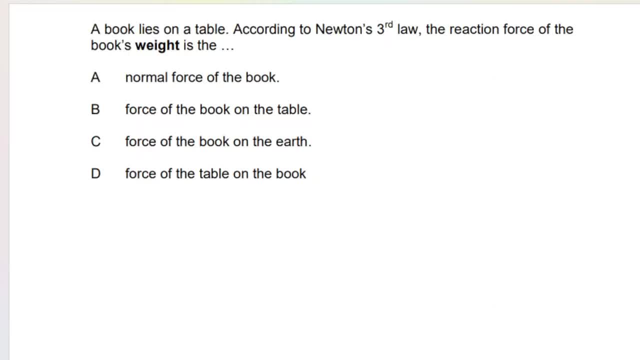 magnitude and the direction of one of the forces. we automatically know the magnitude and the direction of the other force, So I want you to try this past paper question. A book lies on a table. We did this one. According to Newton's third law, the reaction force of the book's weight is the 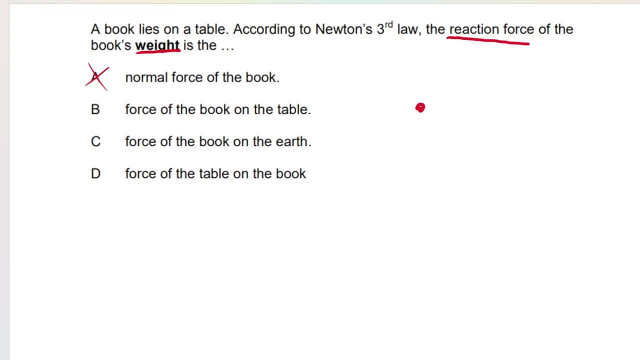 It's not the normal force. Remember we said weight is going straight down, that's Fg. Normal force acts straight up. These two forces are acting on the same object, So that means they cannot be an example of Newton's third law of motion. 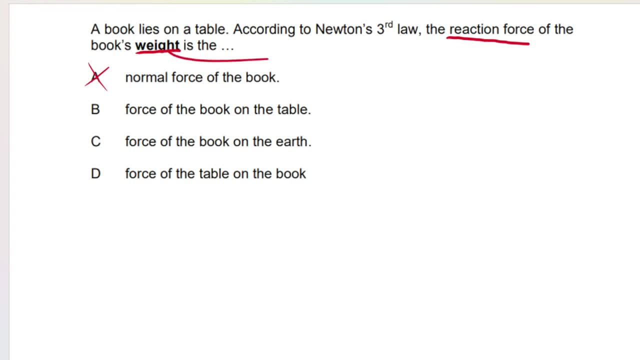 Okay, They need to act on different objects. So the way that you'll do this is: you will work out the fact that weight is the force of the earth on the book, So the one that we are looking for. you need to reverse these words. We are looking 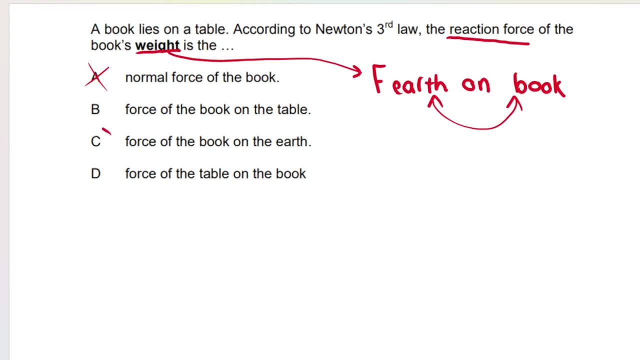 for the force of the book on the earth, We are looking for C. Okay, The table is not in this equation. because we are looking for the force of the book on the earth, We are looking for C. Weight has to do with the object, which in this case is the book and the earth. Okay, So it cannot. 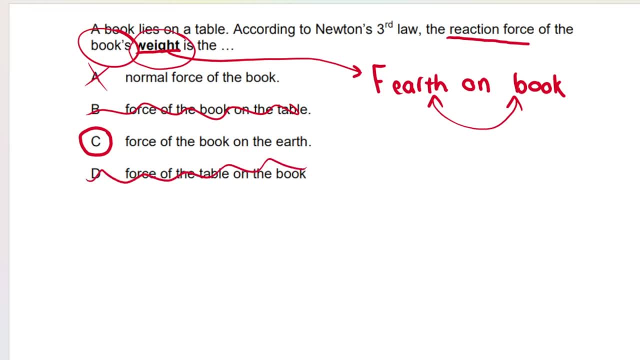 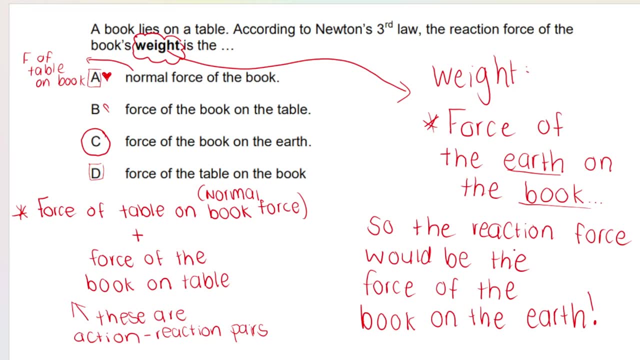 be an option where the table is concerned, And here I've basically just described this in more detail. So I've told you what weight is. So the reaction force would be the force of the book on the earth, which is C. You can see the force of the table on the book. That is the normal force. 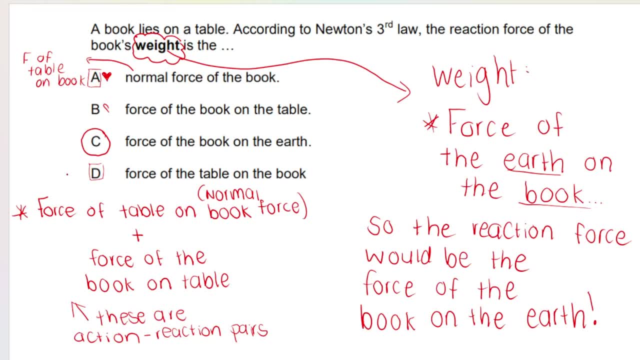 the force of the table on the book, That would be D, The force of the table on the book and the force of the book on the table, Those would be action reaction pairs. Okay, So force of table on book is the normal force. So force of table on book. 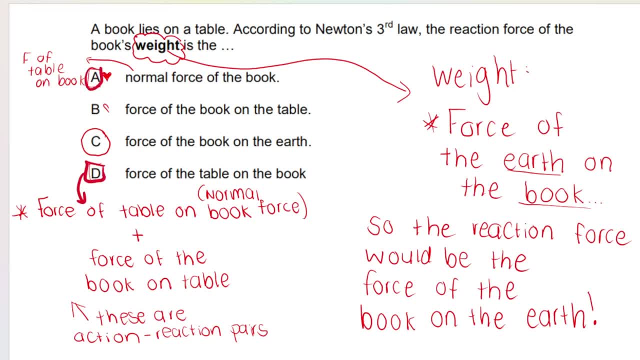 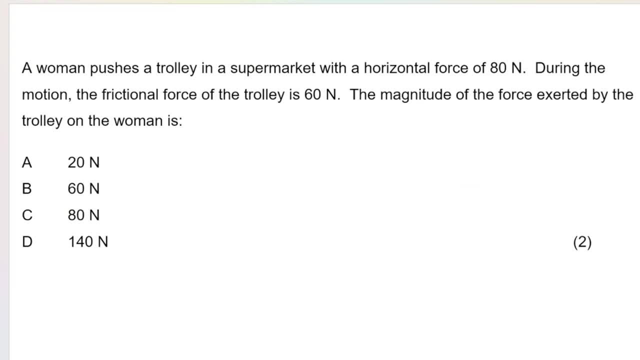 is the normal force. So this and this, technically the same thing, And it's action reaction pair would be the force of the book on the table. So here's another Newton's third law question. A woman pushes a trolley in a supermarket with a horizontal force of 18 Newton. During the motion. 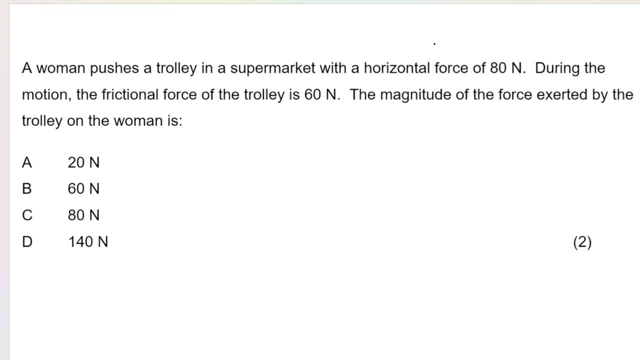 there's a frictional force of 60 Newton. The magnitude of the force exerted by the trolley on the woman is: now they're trying to confuse you. They're not asking you for the net force on the trolley. Okay, So there's a 18 Newton force. Let's say the woman's pushing it to the 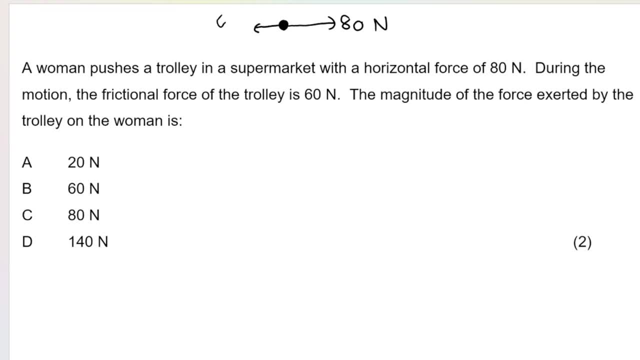 right, And then there's a frictional force in the opposite direction. If they were asking you what the net force is on the trolley, you would say 20 Newton. but they're not asking you for that. They're saying the woman, the force. 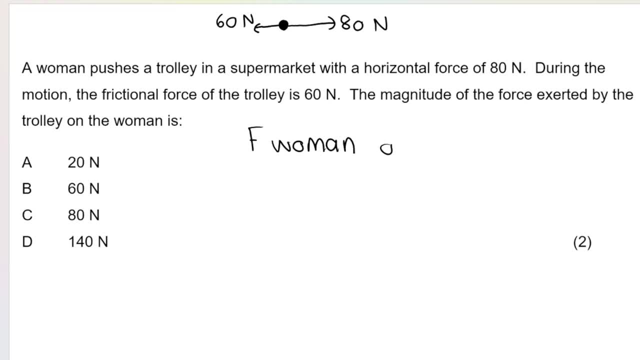 of the woman on the trolley. That's what the question gave you. Read carefully: A woman pushes a trolley with a force of 18 Newton. So the force of the woman on the trolley is 18 Newton. So the force of the trolley on the woman, which is what the question is asking you for. 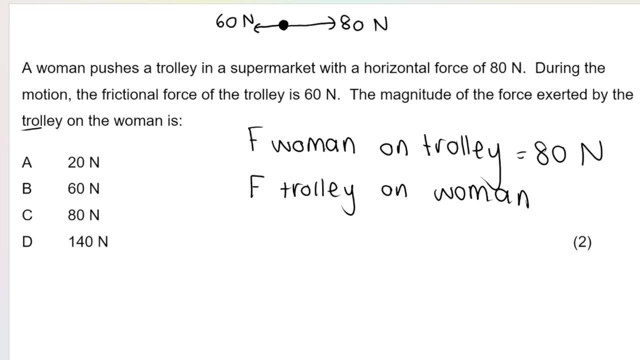 Okay, Of the force exerted by the trolley on the woman, trolley on the woman, woman on the trolley. We reversed the words, So it should also be 18 Newton. There we go, It'll just be in the opposite. 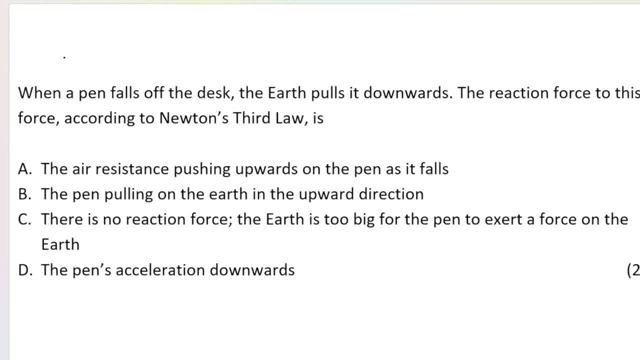 direction. Here's another one for you to try. When a pen falls off the desk, the earth pulls it downwards, Obviously. that's why the pen falls off and moves towards the ground. So they want the reaction force to this force, according to Newton's third law. So remember what we. 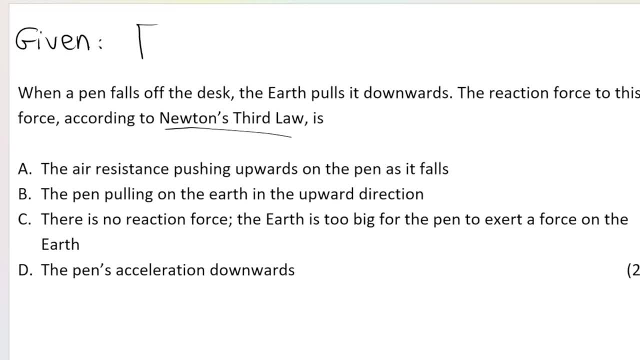 are given. So what the question is giving us is the force of the earth on the pen. So the reaction pair would be the force of the pen on the earth. Which one corresponds to pen on the earth? It would be this one, And I know that sounds weird to you: The pen pulling on the. 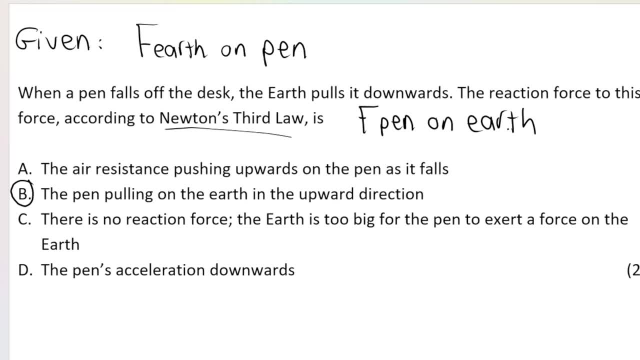 earth in the upward direction. the force of the pen on the earth. You could think, huh, How can a pen pull earth? That is the correct answer, And I know you were probably thinking, ma'am, surely the answer is there's no reaction force because the earth is very big. So how can the pen pull the earth? 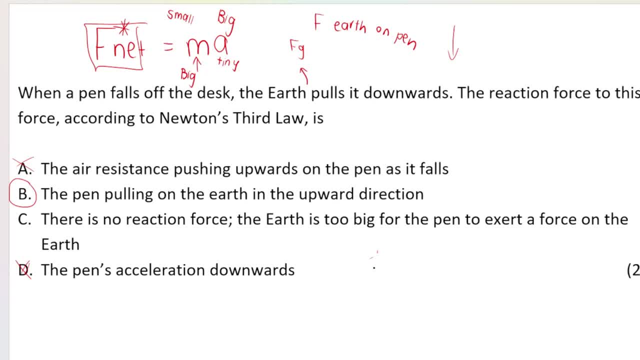 What I want you to think about is the following formula over here, So I'll write it a bit bigger for you: F net is equal to ma. Remember, according to Newton's third law of motion, the force that the pen exerts on the earth is the same force as that the earth exerts on the pen. 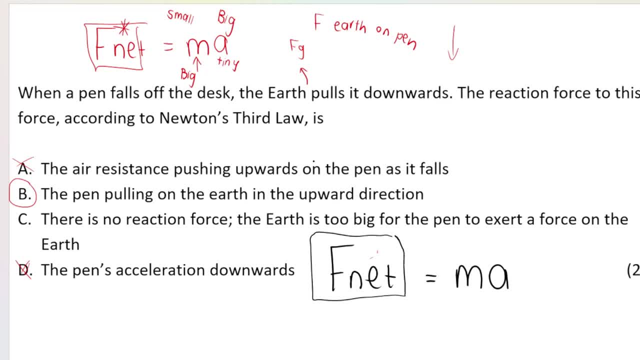 So F net is the same whether we're talking about pen on earth or earth on pen. But because earth has a very, very, very big mass, huge, huge mass. compared to the pen, the acceleration that earth will experience towards the pen is tiny, However, compared to the earth, 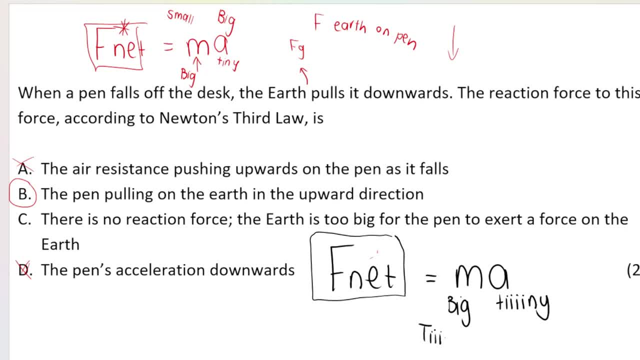 the mass that the pen has is tiny, tiny, tiny, tiny, Very, very small. That means that the acceleration that it will experience towards the earth is massive. I hope that makes sense. That's because of Newton's second law of motion. 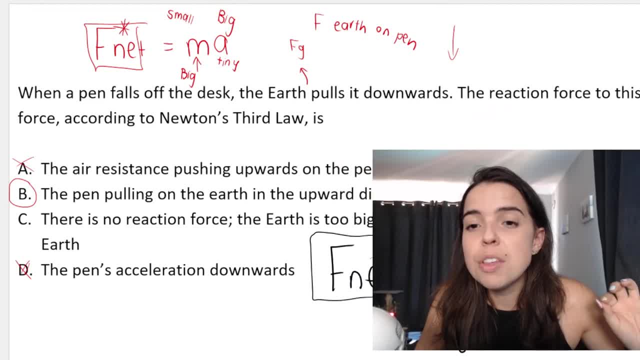 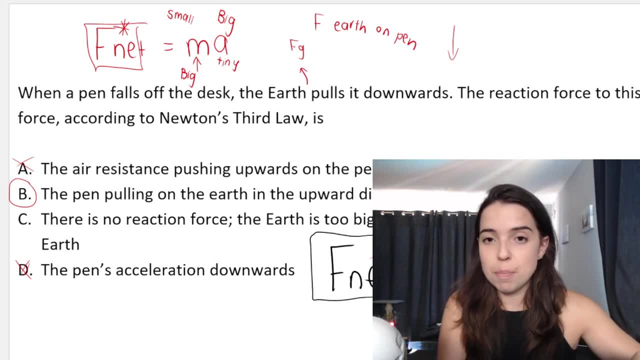 So the force that the earth exerts on the pen- So remember the pen- will fall towards the earth. The force that the earth exerts on the pen and the force that the pen- here's my pen- exerts on the earth, like the planet earth, is the same. 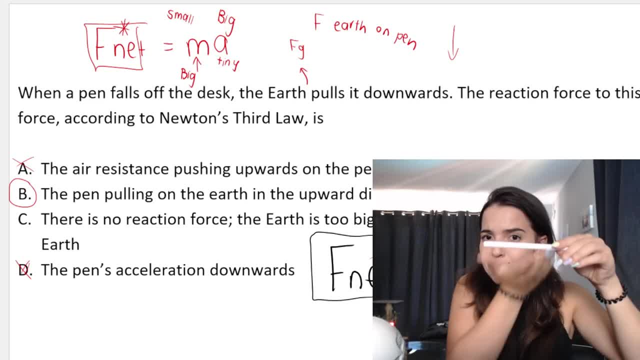 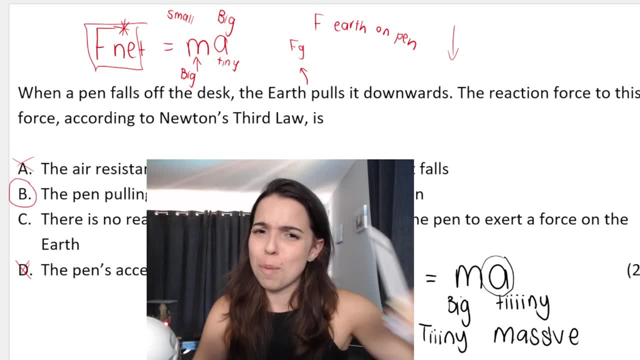 So why is the pen moving towards earth, but earth doesn't move towards the pen? And that's exactly what I showed you over here. It's because the earth has a humongous mass compared to my pen. So therefore, because it has such a big mass, it'll have such a small. 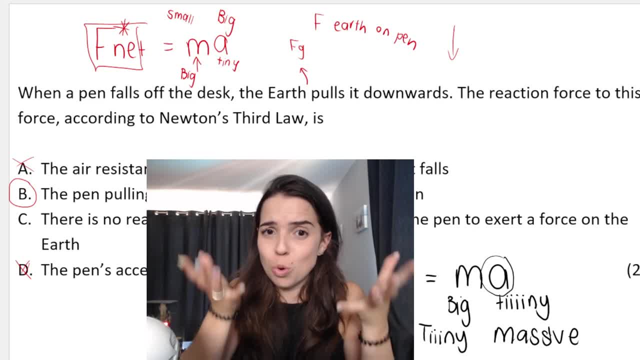 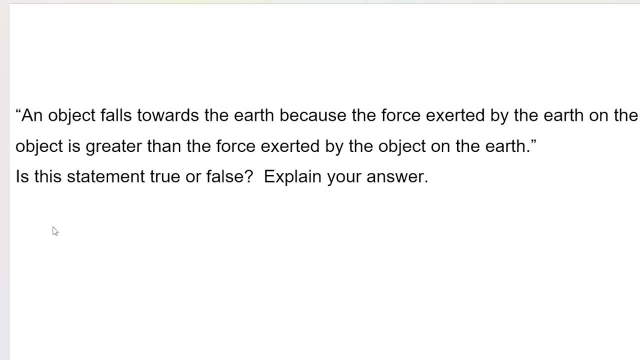 acceleration. We don't even notice the fact that it's moving towards the pen, But because the pen has a tiny, tiny, tiny mass compared to this huge, huge, huge earth, it'll have a big acceleration towards the earth. I hope that that makes sense, And this question over here is testing that exact thing. This comes: 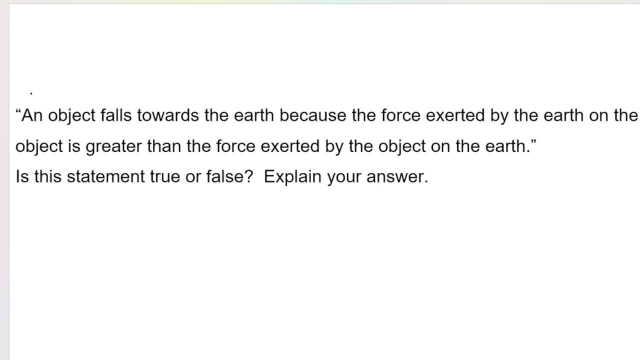 from an exam. So it says: an object falls towards the earth. So here's the earth, Here's my pen. An object falls towards the earth because the force exerted by the earth on the object is greater than the force exerted by the object on the earth. We already know that that is false because of 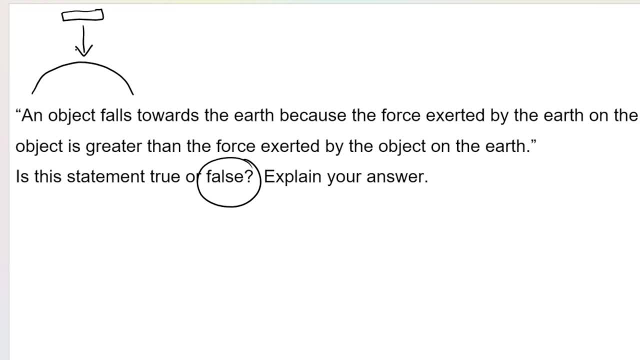 Newton's third law of motion. So, yes, the downwards force that the object experiences, the force of the earth on the pen, which is the weight of the pen. right, That's the weight of the pen, the force that the earth exerts on the pen. But we learned that, according to Newton's, 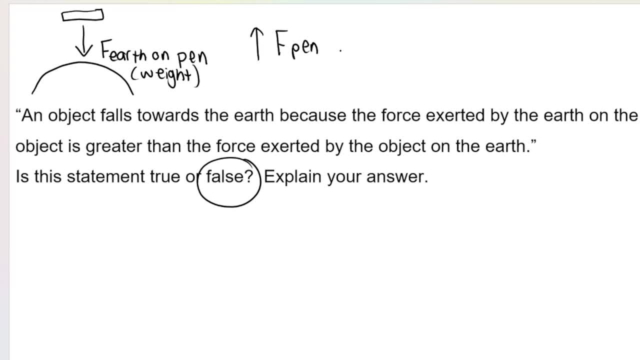 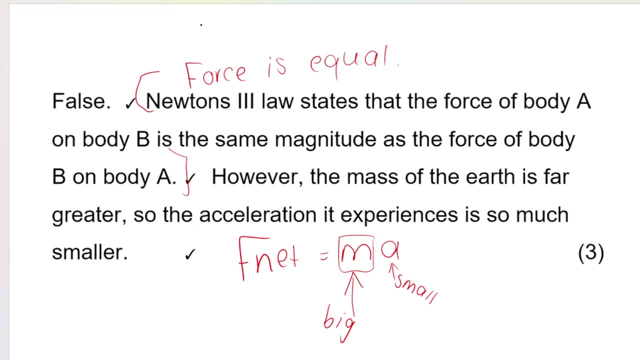 third law of motion, the force that the pen exerts on the earth is of the same magnitude but in opposite directions. So it's false. But why does the pen go towards the earth and the earth doesn't go towards the pen? There's your answer. Newton's third law states that the force 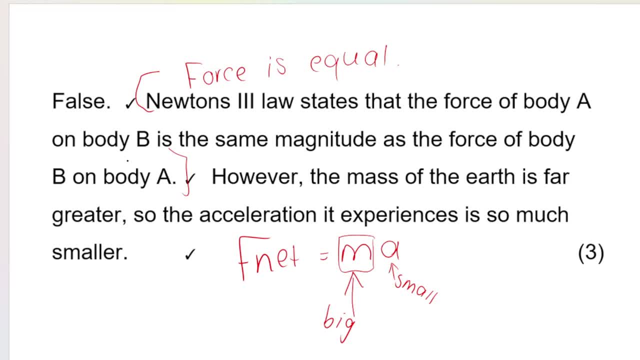 of motion is greater than the force of the pen, So it's false. But why does the pen go towards? the body a on body b is the same magnitude as the force of body b on body a simultaneously. at the same time, however, the mass of earth is far greater, so the experiences a much smaller acceleration. 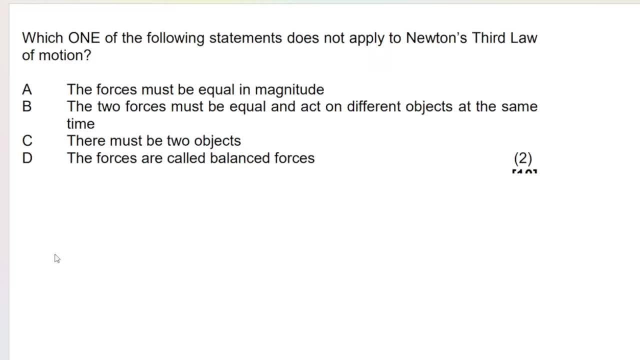 our last newton's third law of motion question. which one of the following statements does not apply to newton's third law of motion? the forces must be equal in magnitude. the forces must be equal and act on different objects at the same time. there must be two objects. the forces are. 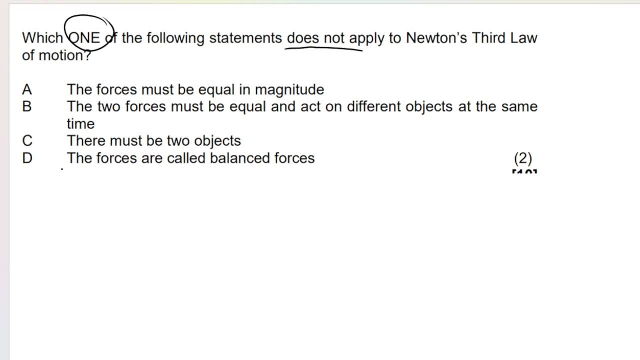 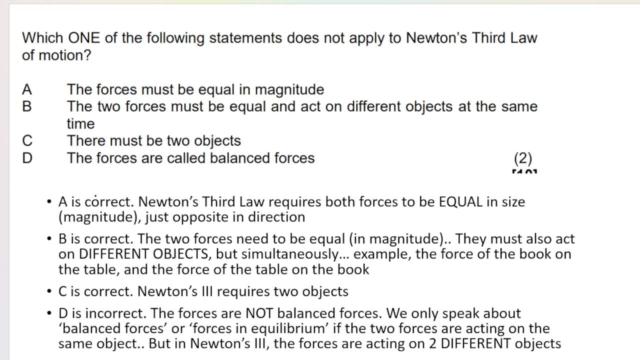 called balanced forces. i hope the correct answer or the following statement that does not apply, screaming out at you: it's this one, remember. a is correct. newton's third law requires both forces to be equal in magnitude, just opposite in direction. b is correct because we have equal. 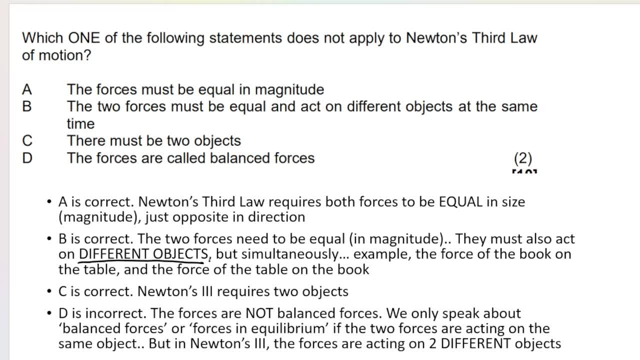 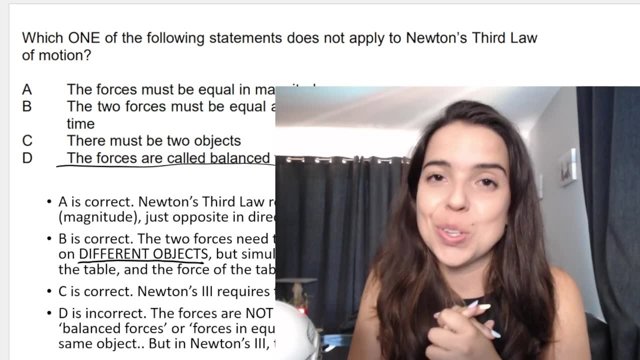 forces but they must act on different objects, like book on table, table on book. t is correct. there must be two objects: table, book, book, table earth, ball, ball earth. but d is correct because they are never considered balanced forces. i hope that this video has helped you understand newton's third law of motion a little bit better. they can definitely. 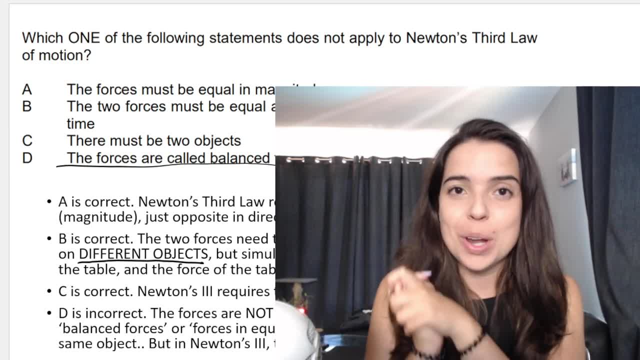 try and trick you with the multiple choice questions and i hope to see you in more newton's law videos, more physics, more chemistry. can't wait to see you guys in the next video. subscribe for more. bye everybody.